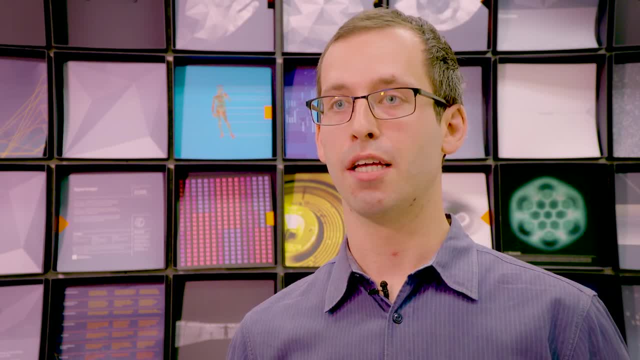 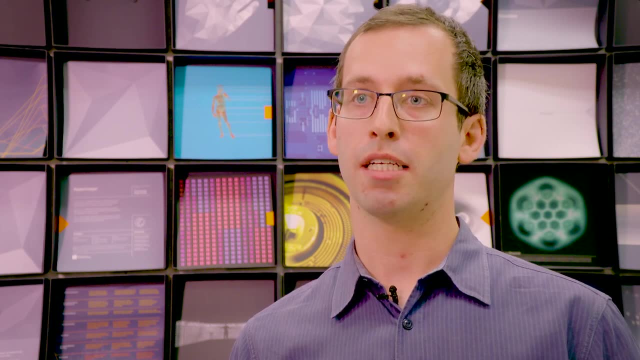 held up for about 50 years. but we now understand that there's one exception to this rule, And the exception is quantum computers. Quantum computers use a fundamentally different instruction set than classical computers. As a result, they can run different algorithms and they 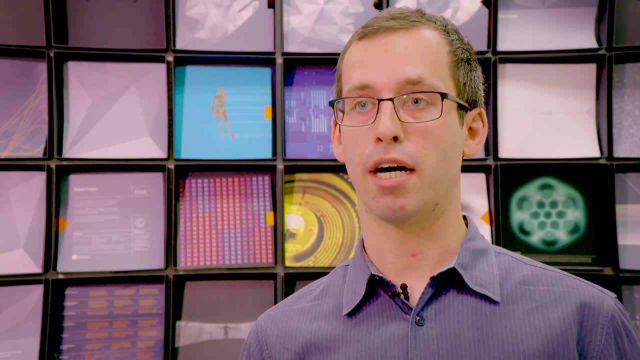 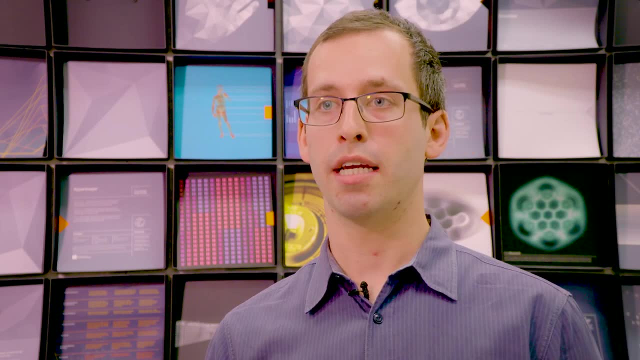 can run algorithms you could not run on classical computers. Those algorithms make use of quantum effects like nonlocality, entanglement, superposition and interference, And so when you're designing a quantum algorithm, your aim is to exploit those quantum effects to make you get the 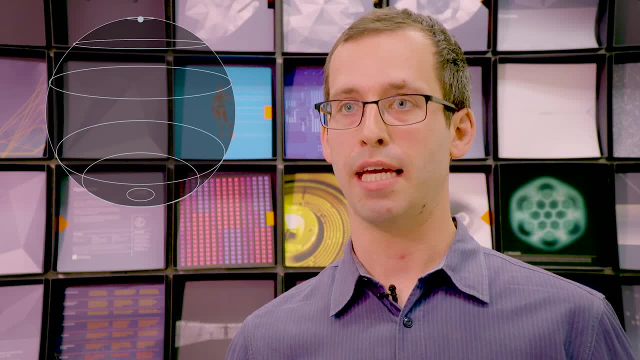 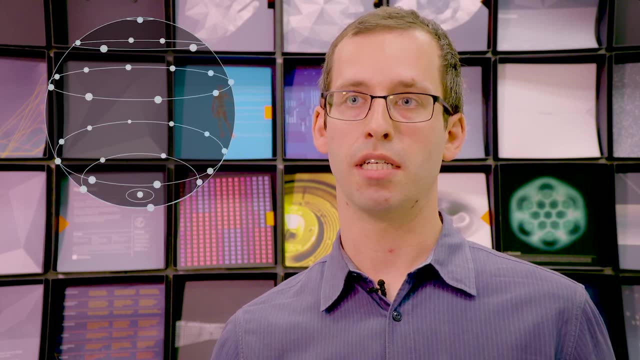 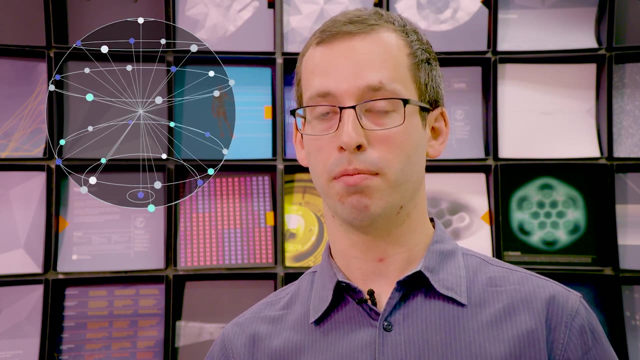 solution faster. Generally speaking, an algorithm might start by taking your classical input to the problem, processing that into a quantum state which is a superposition of an exponential number of classical states. Then you aim to transform that quantum state, which encodes the problem, into a quantum 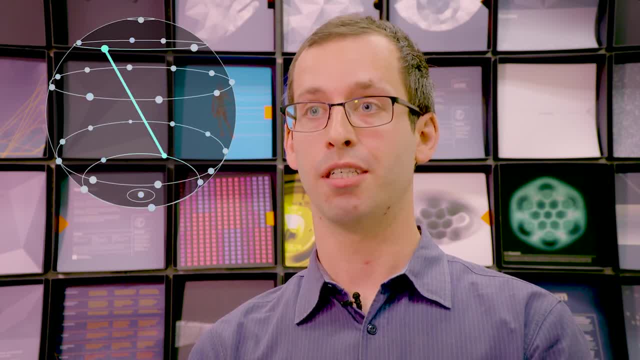 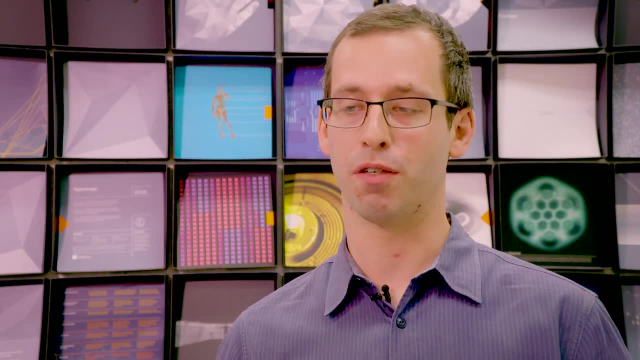 state which encodes the solution, And from that quantum state you measure and you get the solution. Now, of course, to make this work, it's a bit of an art and you have to design an algorithm which follows these steps for a given problem And some of the areas.